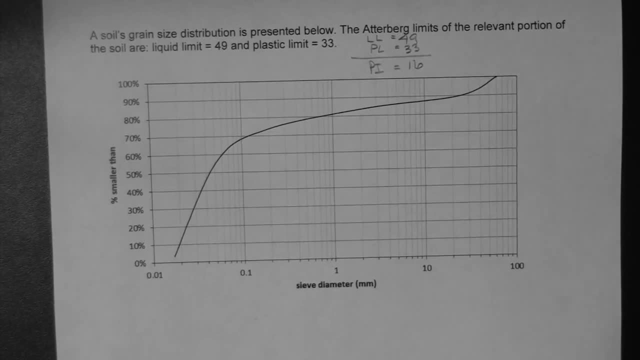 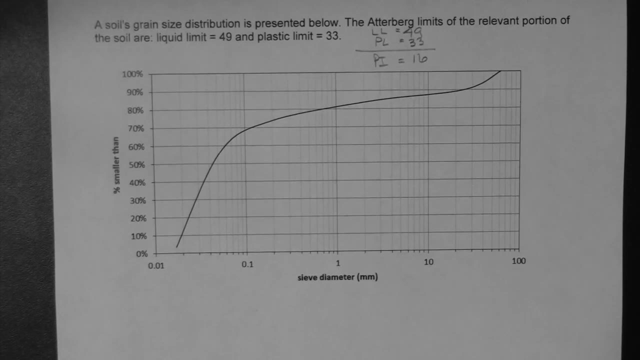 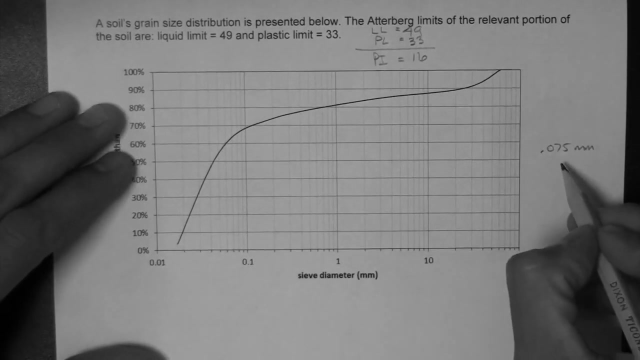 is that we have to find the percentage of fines. So the percentage of fines in our soil is the percent of the soil, that is, of the mass of the soil that is composed of grains smaller than 0.075. Millimeters, right? 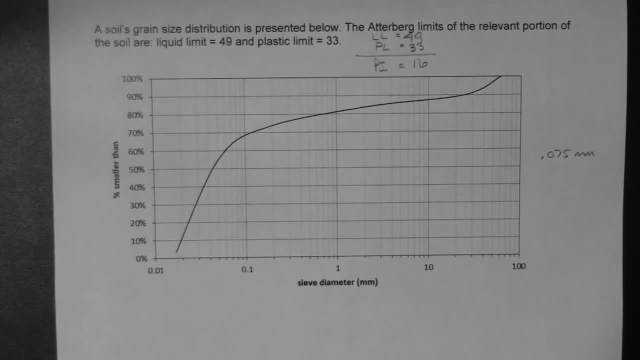 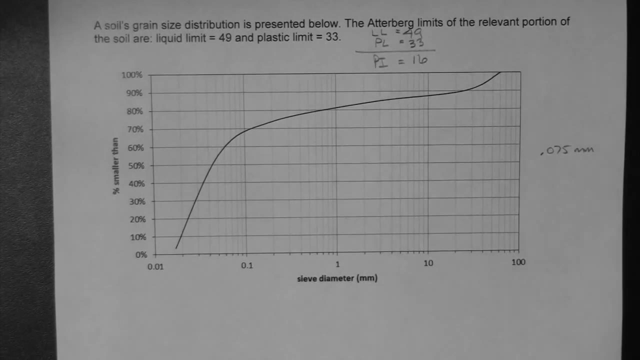 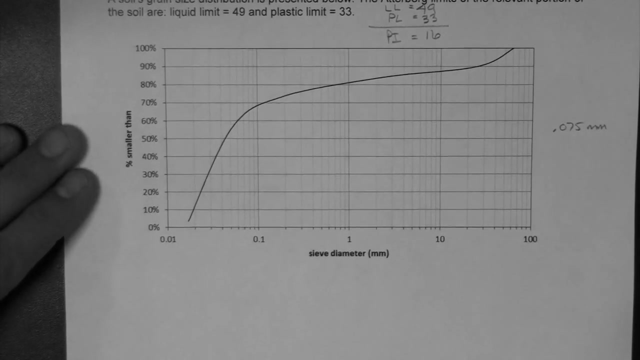 Less than 0.075 millimeters. that is, if the diameter is smaller than this, the particle is fine, And if the diameter is larger than that, the particle is coarse. Okay, so how do we do this? Well, we go here to the log scale and we read where the 0.075 millimeter mark is. 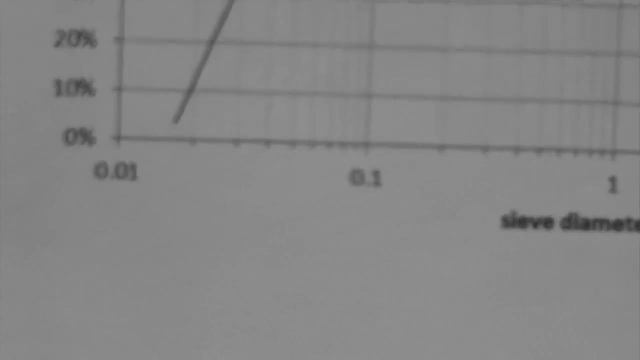 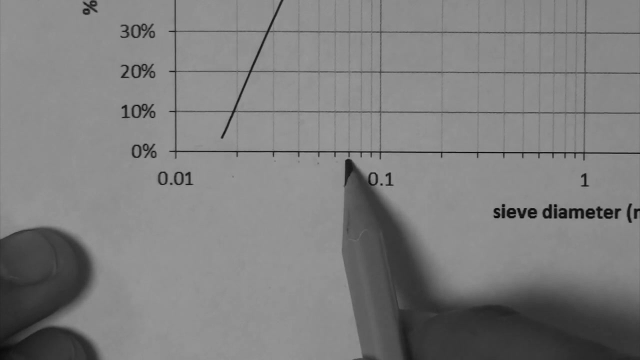 So let's zoom in: 0.01,, 0.02,, 0.03,, 0.04,, 0.05,, 0.06.. 0.06, 0.07, 0.08.. 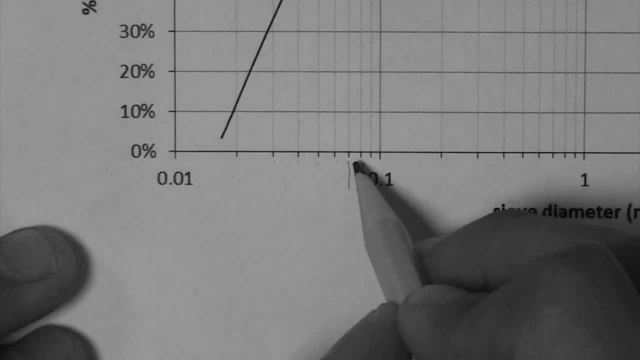 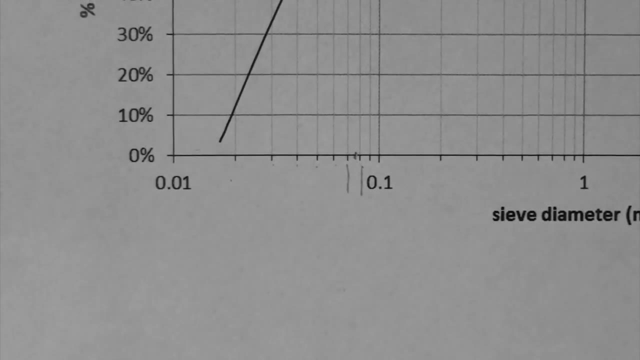 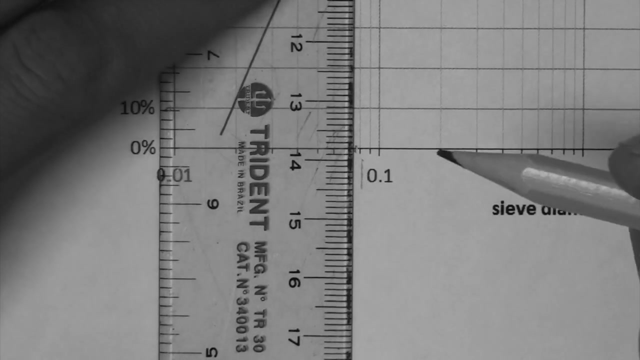 0.07 and 0.08, right, 0.07 and 0.08.. So 0.075 is not at the center, but a little bit to the right. Okay, And remember we are approximating, so to be close enough is okay. 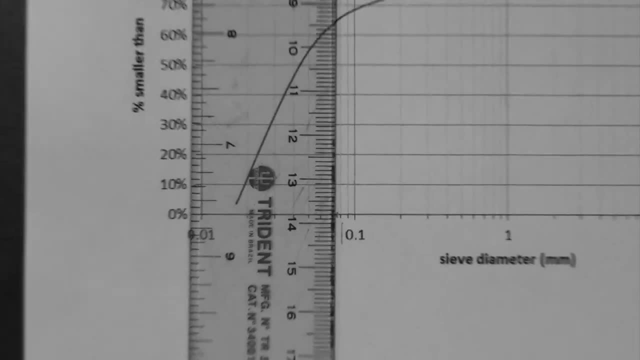 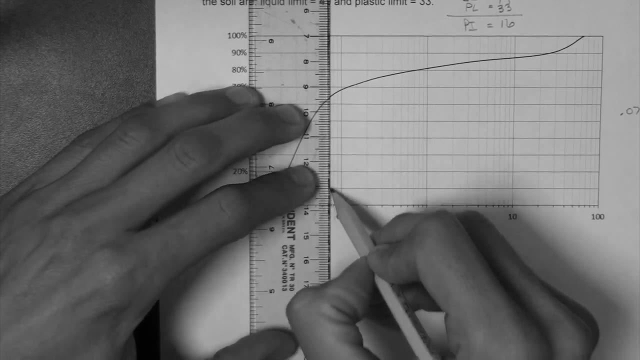 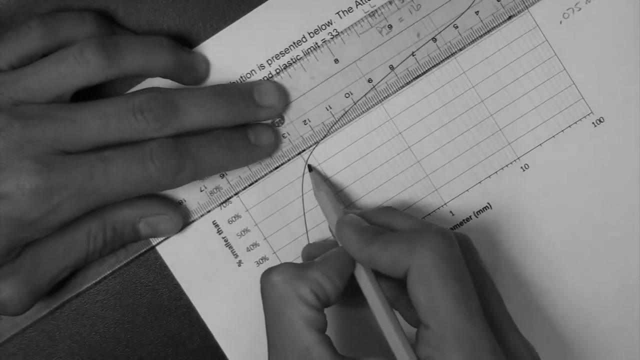 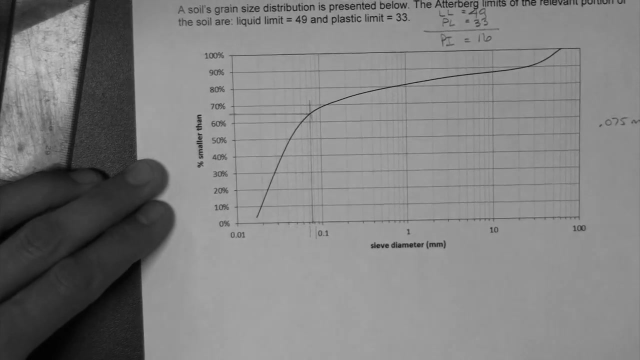 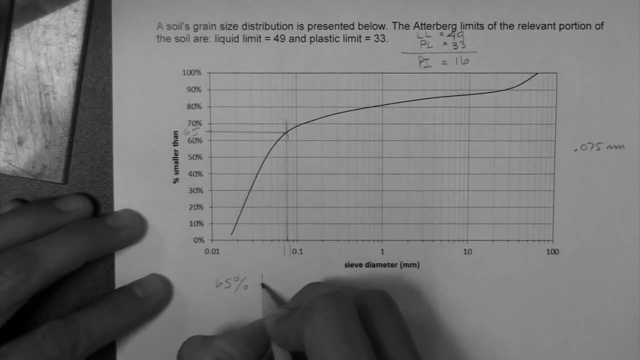 Alright. so now what we do is we take that point and we draw a vertical line up until it touches our greenhouse distribution, Okay. And then we read the percentage: 65%. So our soil is 65% fines, Right. 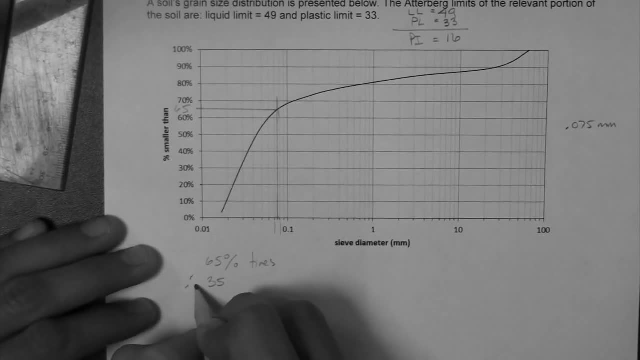 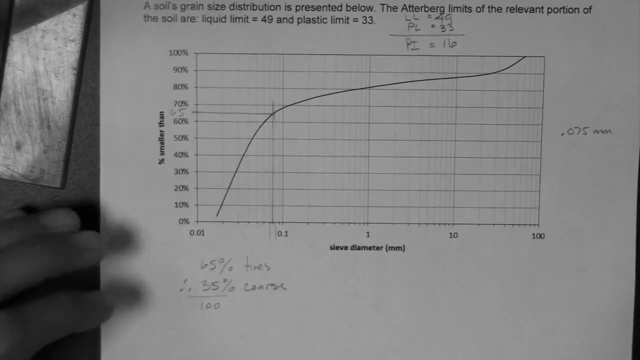 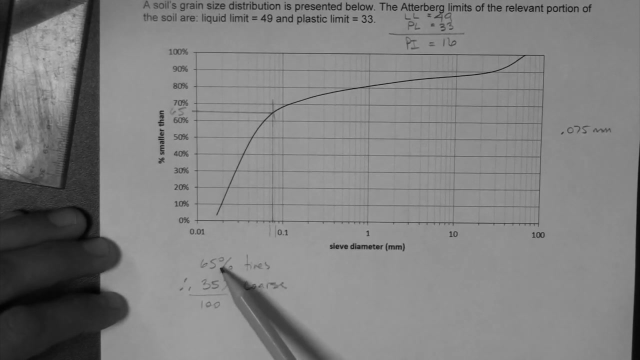 And that means that 35%. so therefore 35% this makes 100. obviously is coarse. Okay, very simple. So we have more fines than coarse, Right? The fines content is more than 50%. This is the fines content. 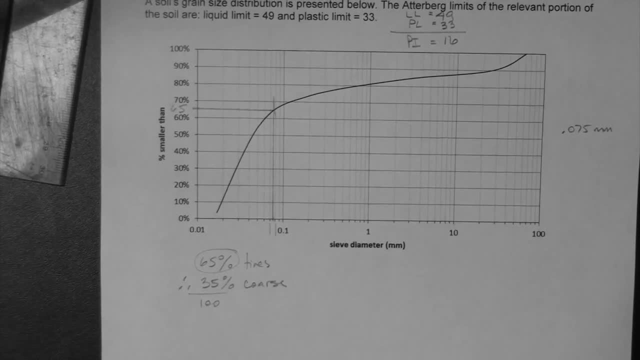 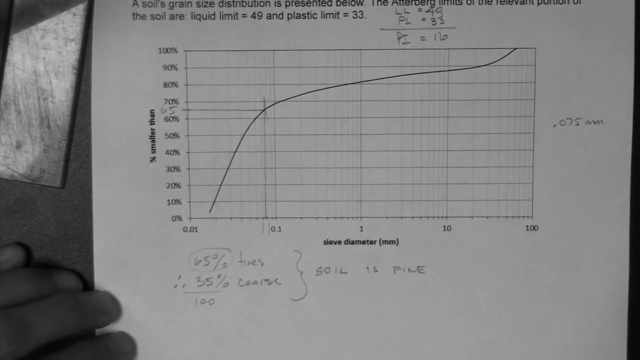 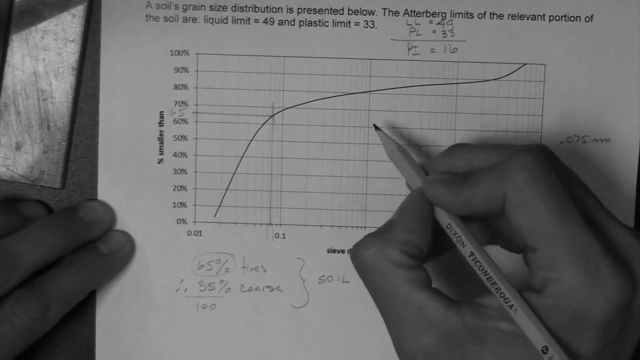 60%, 65%. It is more than 50%. therefore, our soil is fine. The soil is fine-grained, even though it has coarse grains in it. Okay, That's this side of the greenhouse distribution. This is the coarse portion. 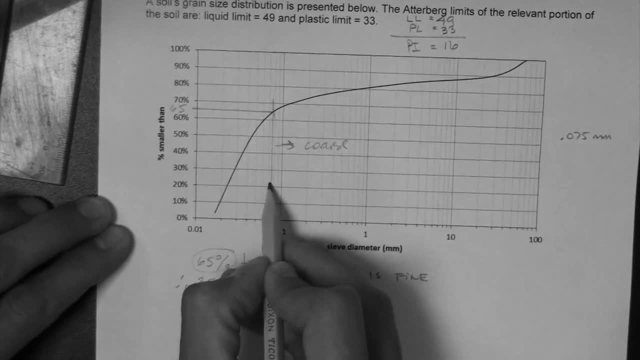 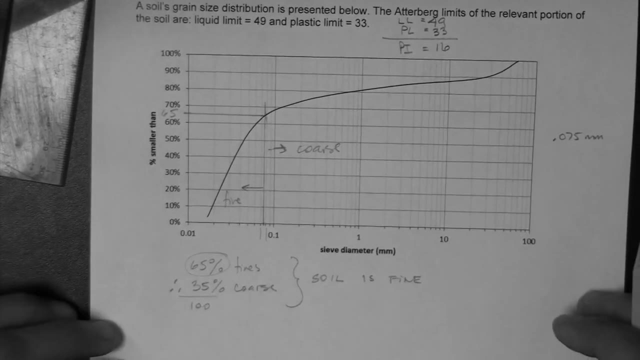 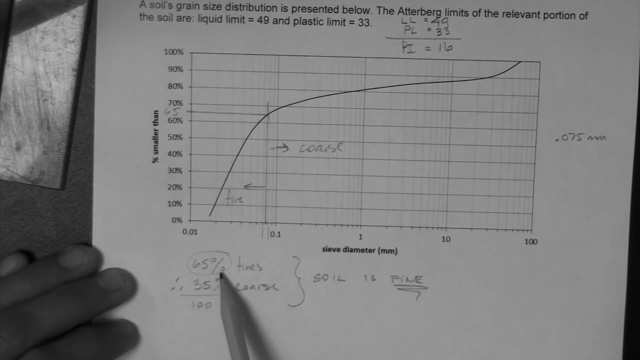 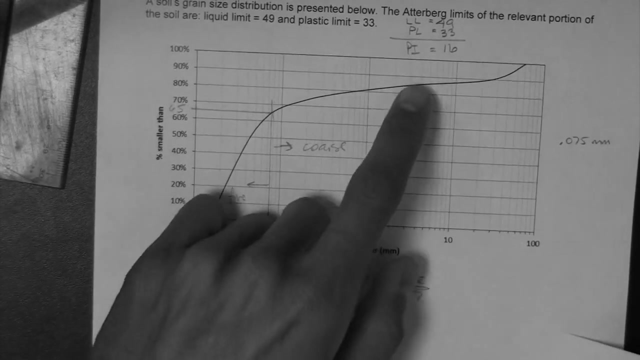 This way And from here, fine portion. Okay, So what do we do if the soil is fine? If the soil is fine because more than 50% of the soil is composed of fines, then what we do is we simply utilize our liquid limit and plasticity index. 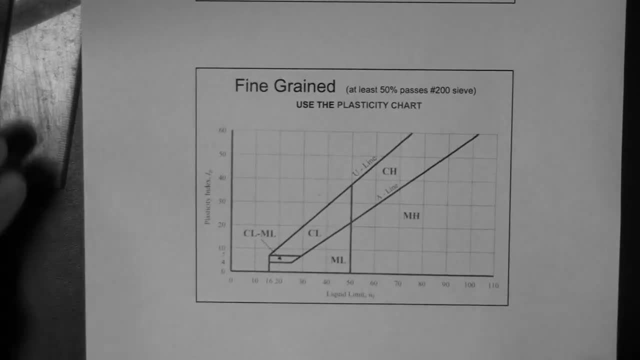 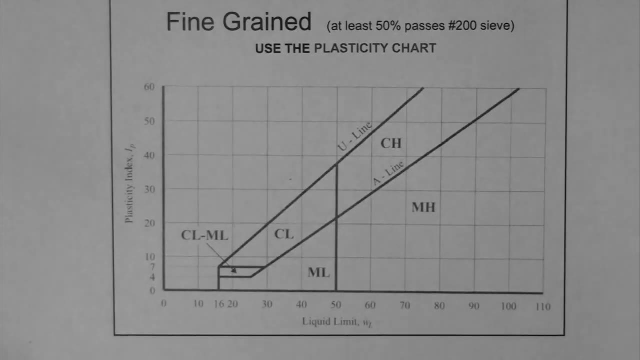 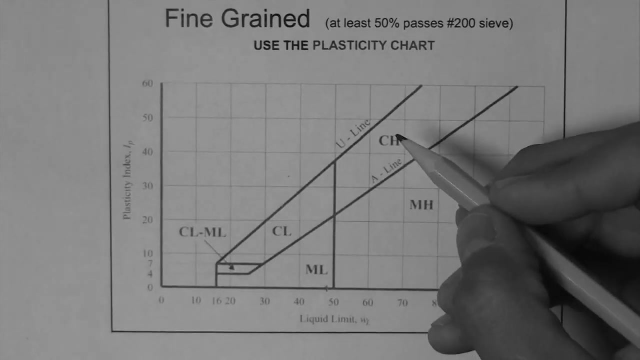 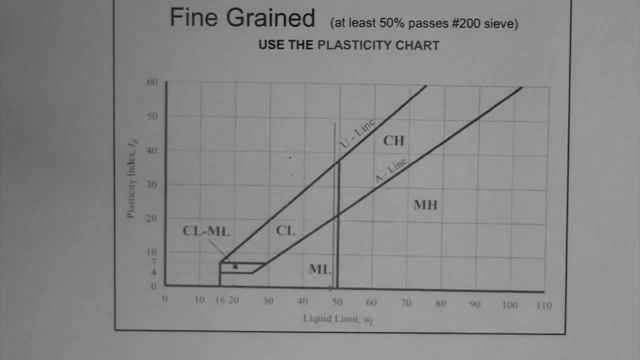 and map those numbers on the plasticity chart. Okay, So our liquid limit was given as 49. This is 50,. 49 is here, right, We can draw a vertical line there, And our plasticity index is 16.. 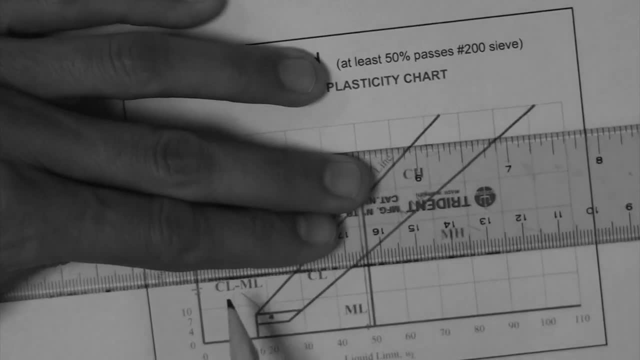 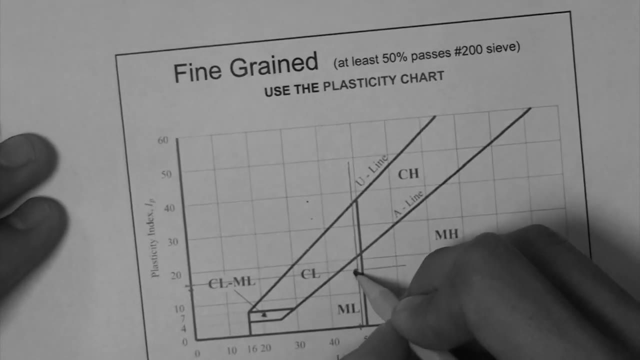 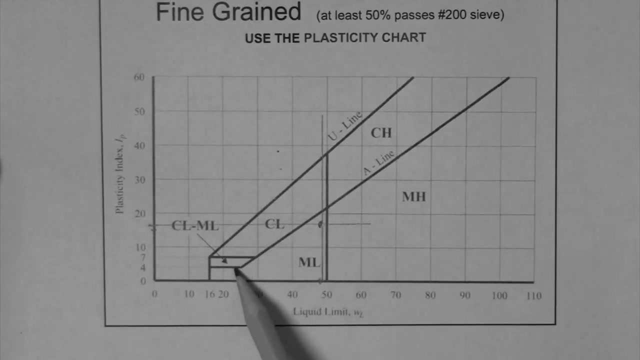 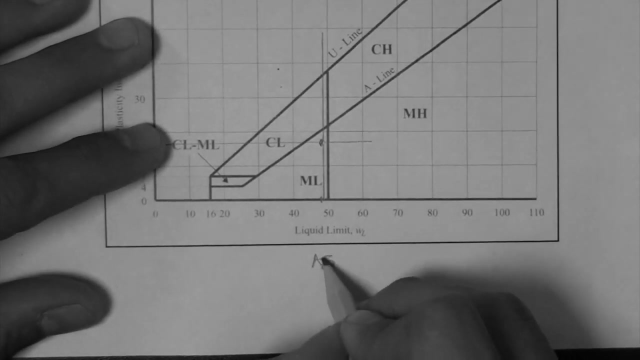 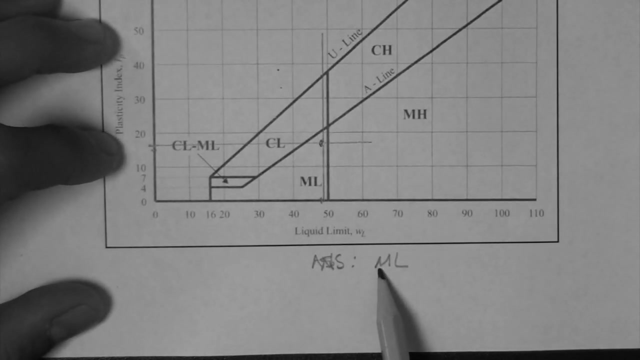 This is 15,, 16 is there. So our point lands right there. It lands in the region called ML. That means that our soil- the answer oops. the answer is that our soil is an ML Low plasticity silt. 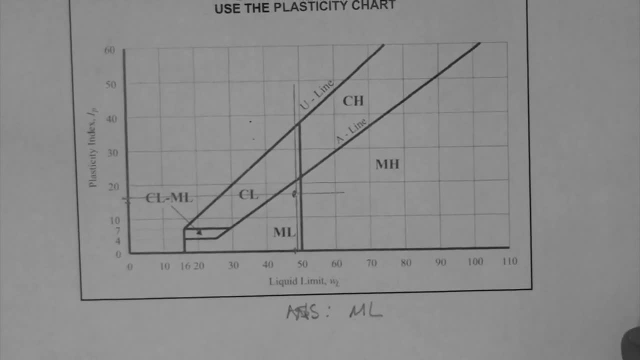 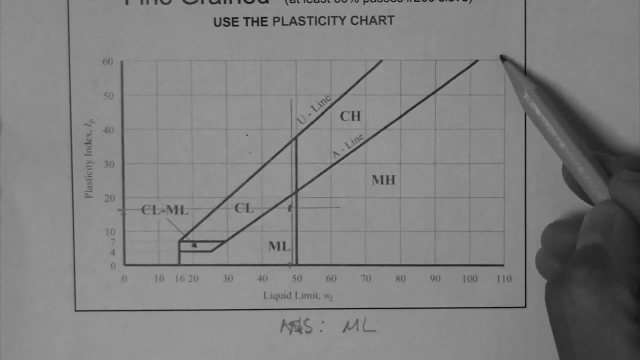 Okay, Now just for completeness here. if our soil point had landed somewhere over here in this region, this would be a high plasticity silt In this region here, high plasticity clay In this region, low plasticity clay. 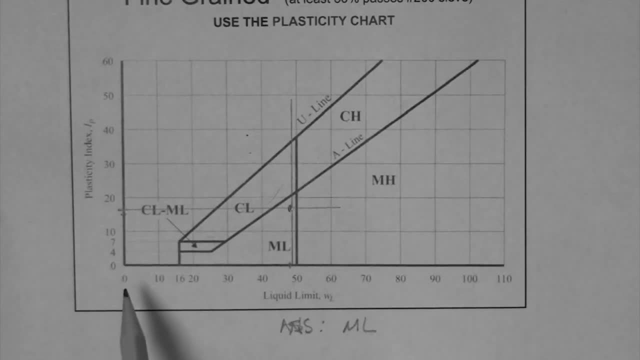 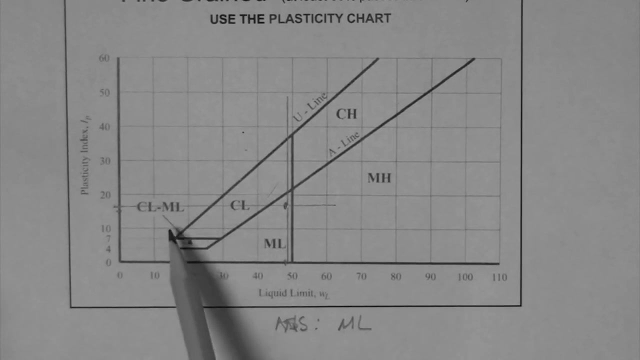 And in this small little region here it's called a CLML, which means that it is a soil that behaves somewhat in the middle, let's say, between CL and ML, meaning that it has some CL-like properties and also some ML-like properties. 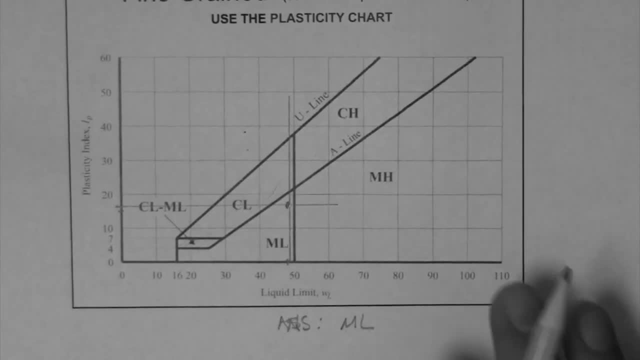 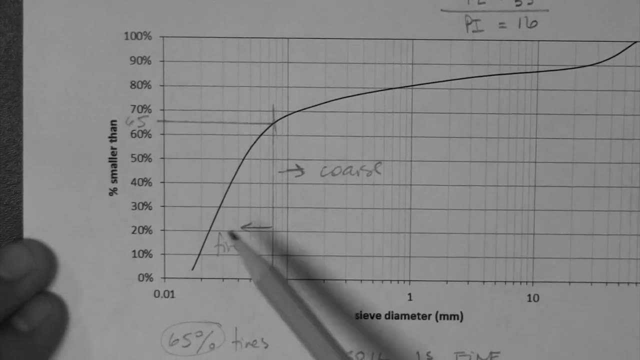 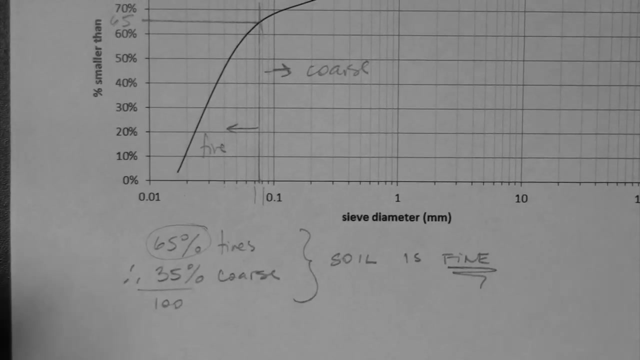 That's this little region here. Okay, But notice again, if the calibric limits were given for the finer portion, we found that the percentage of fines is more than 50,- 65% in this case, meaning that we can neglect the rest of the grain size distribution.